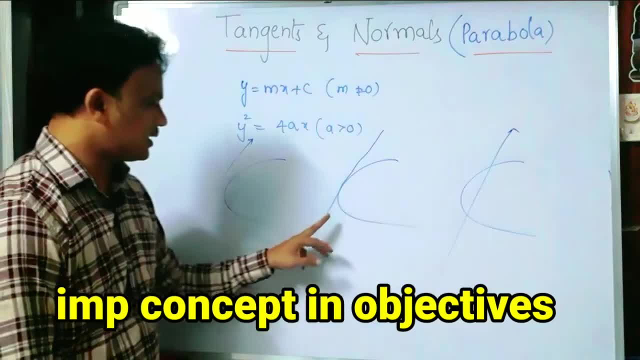 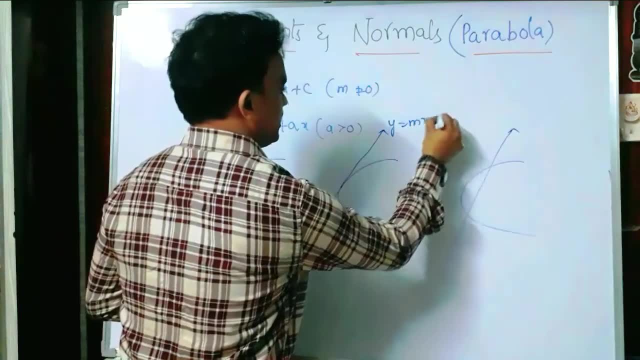 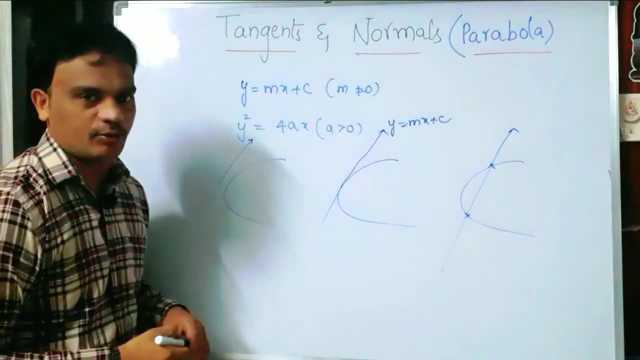 may touches the parabola, may intersect the parabola. In this case we can say: the line y equals to mx plus c. Yes, the line y equals to mx plus c is a tangent, So in that case it is a secant. Okay, in that case it not. it is not intersecting the parabola, So in that case, 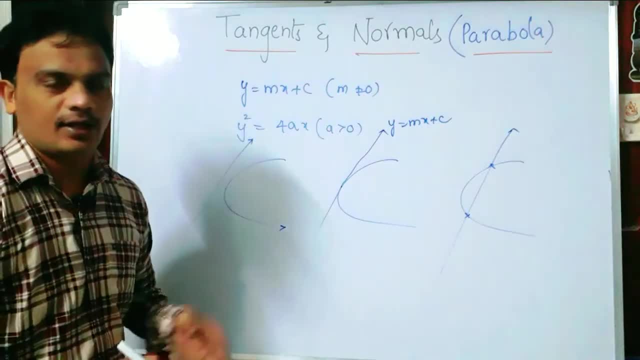 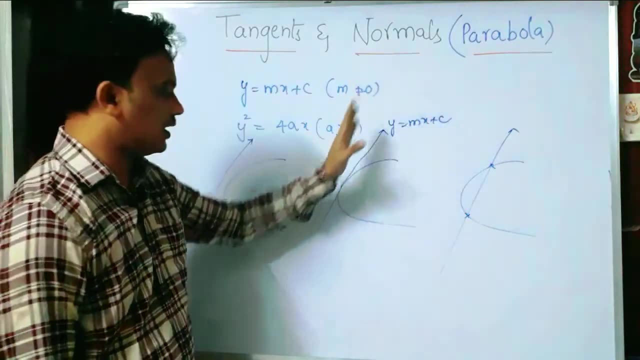 what are the conditions? We are going to discussing that, Okay, yes. what my topic is? the line y equals to mx plus c is a tangent to the parabola. In that case, what are the conditions? That one, Okay, yes. first of all, I am going to finding the point of intersection of the line y. 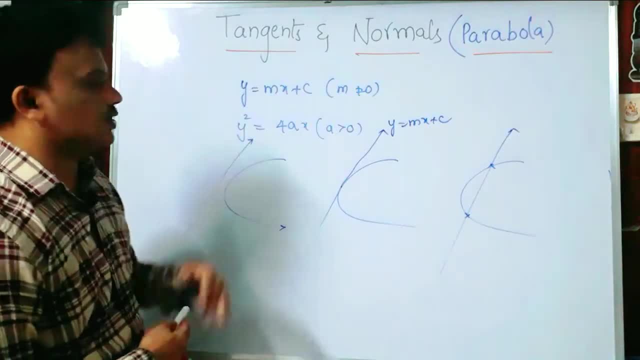 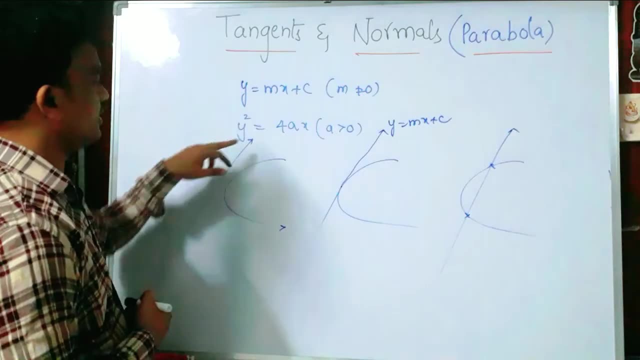 equals to mx plus c. the given parabola, y square is equals to 4ax. Yeah, what are those? Come on, let us see. Yes, So y equals to mx plus c, So that y values are substituting in the parabola. 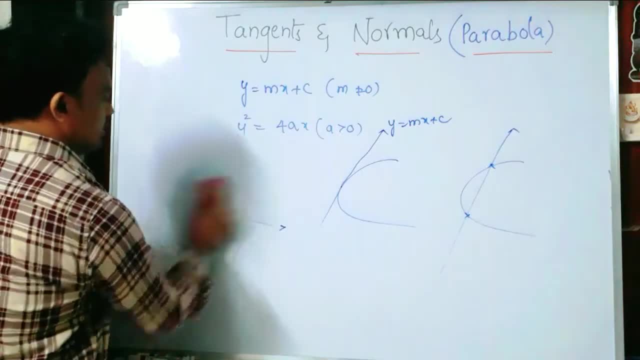 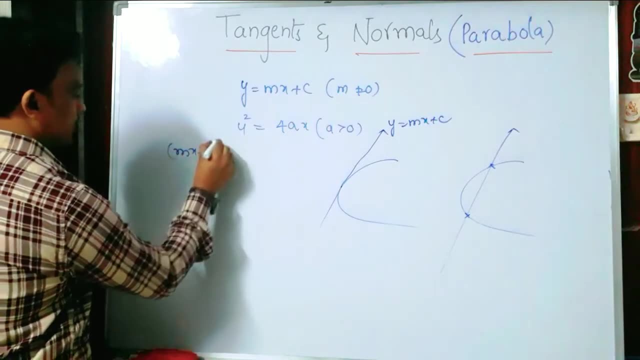 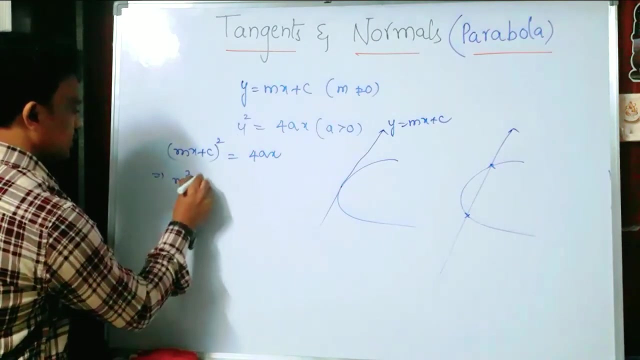 y square is equals to 4ax. What you can get. Yeah, let us see here I am explaining that Y square, which is mx plus c whole square, equals to 4ax. Okay, yes, So it is m square, x square. 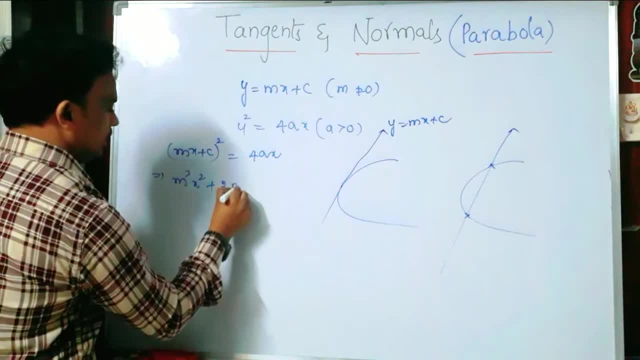 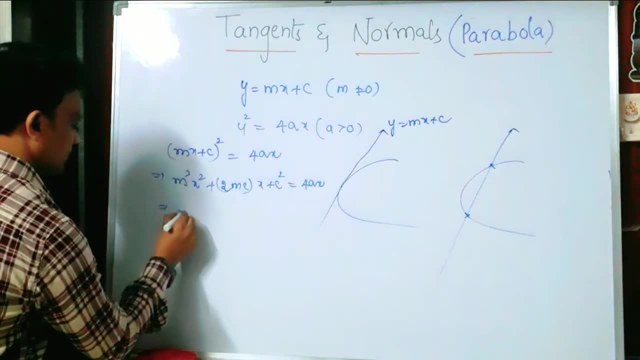 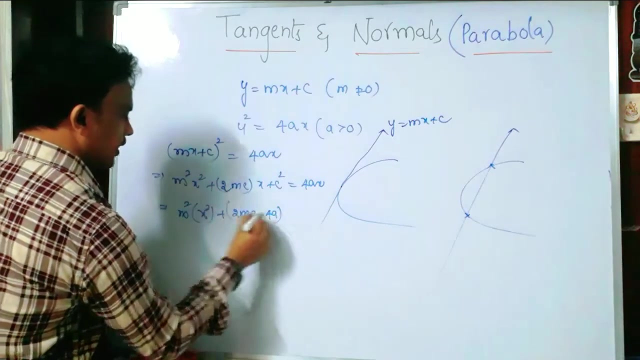 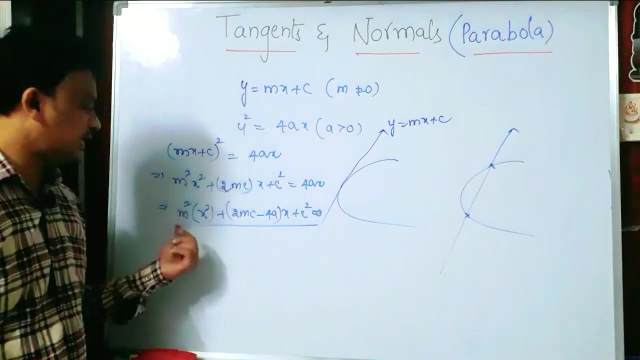 plus it is 2mc into x plus c square equals to 4ax. Okay, yes, simplify the terms: m square of x square plus 2mc, minus 4a of x plus c square equals to 0.. Right or not? So here we got the second degree equation in terms of 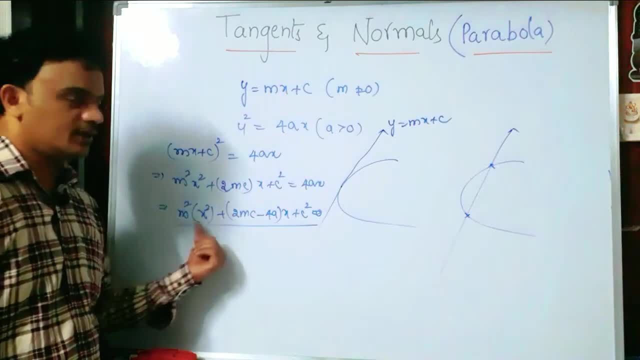 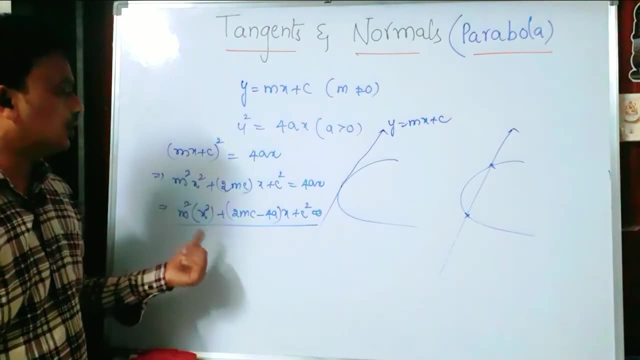 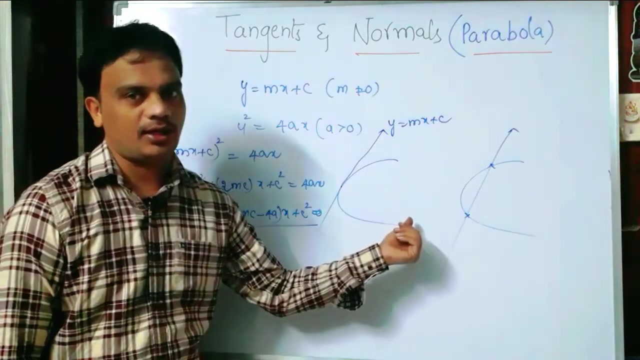 second degree equation in terms of x square, Right or not? Second degree equation in terms of x square. Okay, yeah, So if it is a circle, if sorry, if it touches the parabola, if it touches the parabola, then for this quadratic equation in terms of x square. 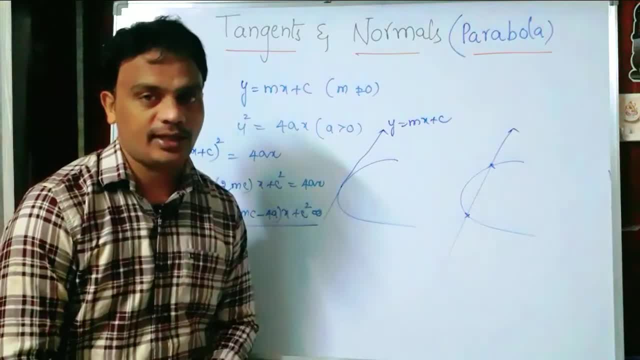 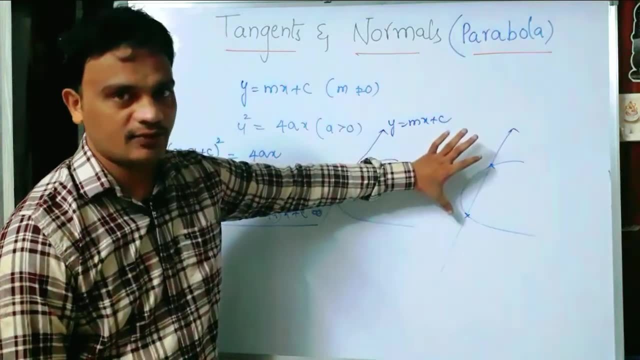 right. the delta should be equals to 0.. Am I right or not? If it intersects that the parabola it touches, it intersects the parabola. it has two distinct values of x. Okay, So in this case, 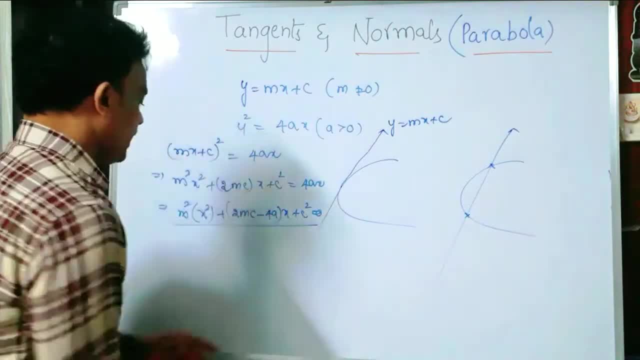 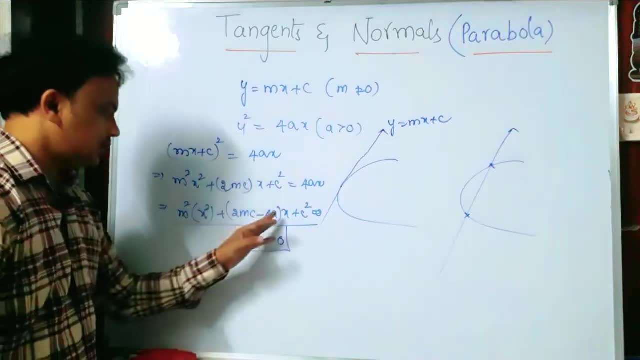 delta becomes 0, it touches at only one point. So here I can say the delta. if delta is equals to 0, if delta is equals to 0, that means for this quadratic equation okay. so if delta equals to. 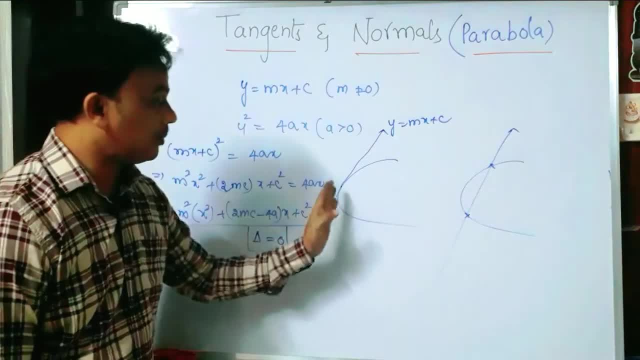 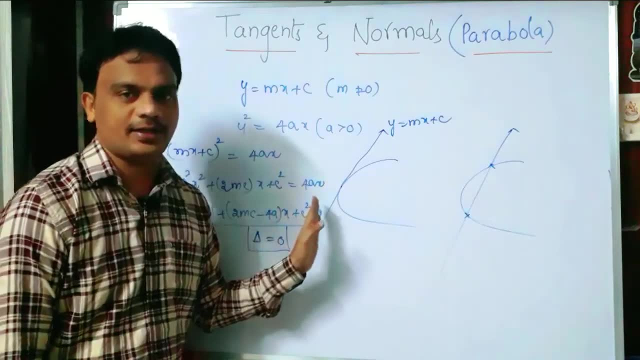 0, that means. so this line touches the parabola at only one point. I mean the point of intersection is one point. That means roots are equal. There are no two distinct points. In that case, the delta equals 0.. Come on. 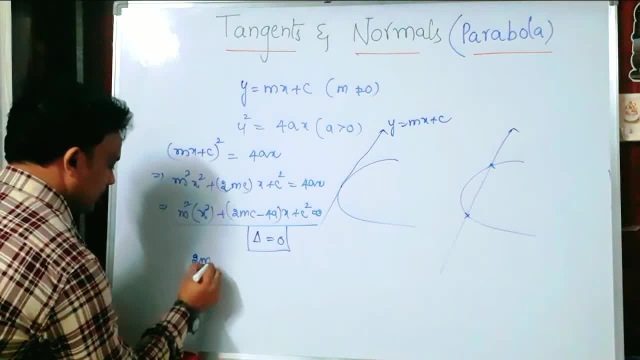 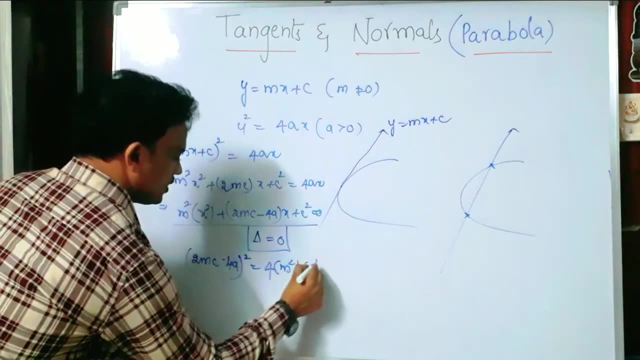 please find out the delta. So b square, which is 2mc minus 4a, whole square, b square equals to 4ac, 4 into m square, into c square, 4a and c. Okay, come on, simplify this one. take out two common 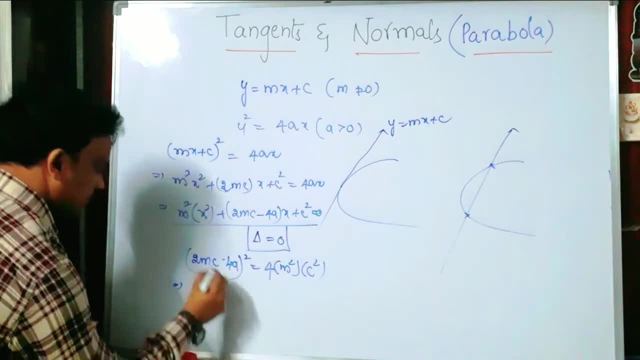 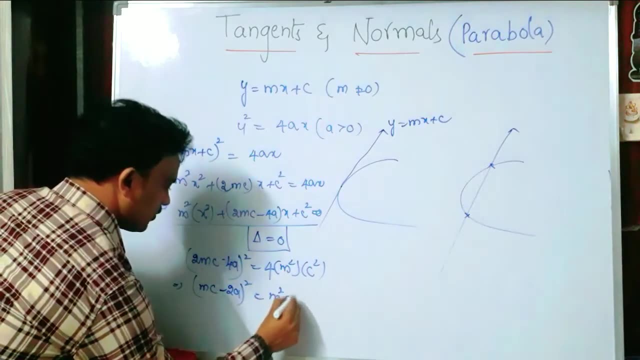 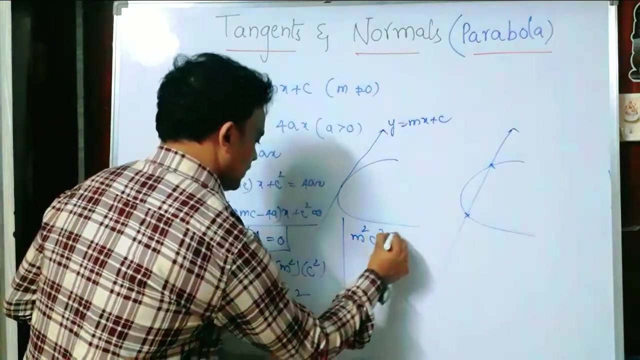 and the squaring four, both sides cancel. which is mc. Okay, which is mc minus 2a, whole square equals to m square and c square. Okay, yes, come on simplifying this term. So which is m square, c square, m square, c square plus 4a square. 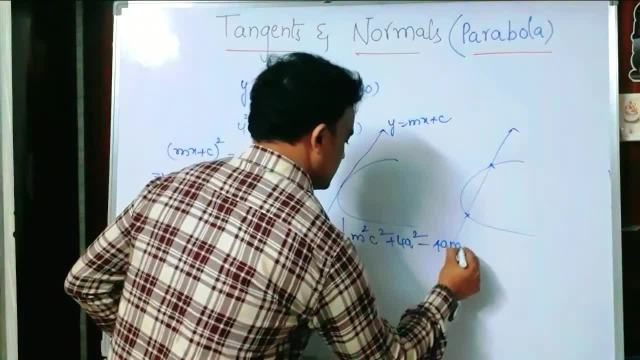 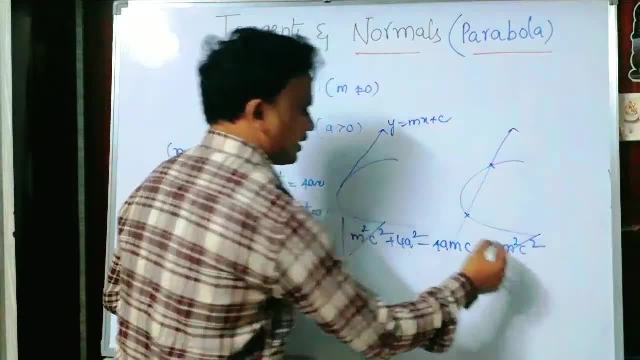 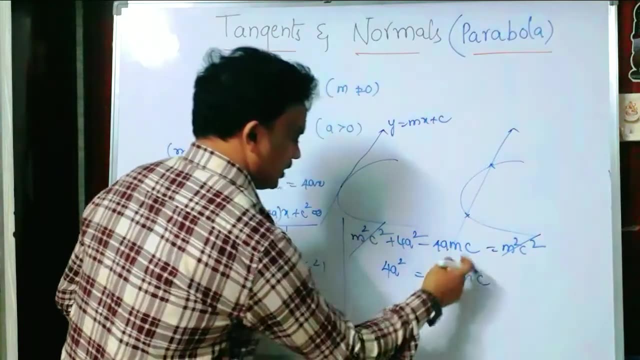 4a square minus 4amc. minus 4amc is m square and c square. Yes, both sides m square, c square get cancelled. Okay, So which is 4a square is equals to 4amc, 4a, 4amc, both sides of 4a, 4a get cancelled. 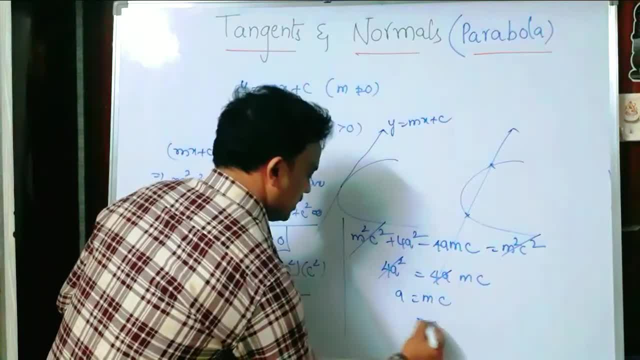 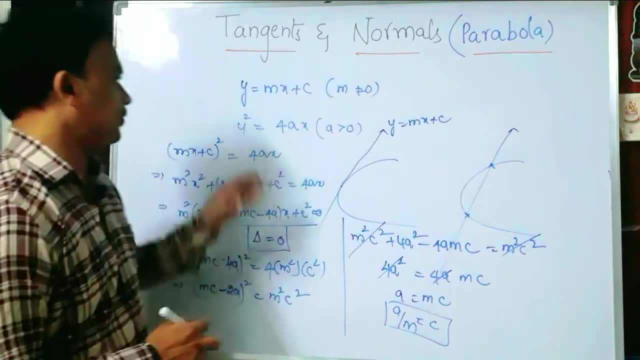 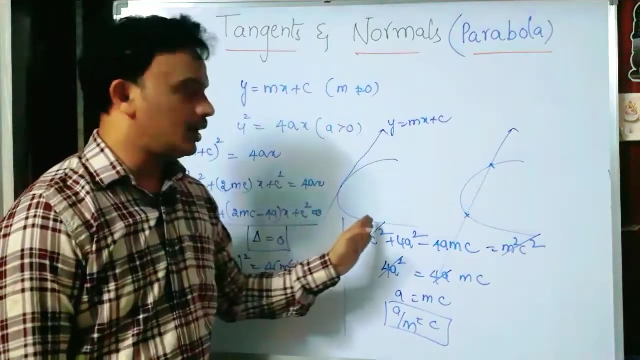 Okay, then a is equals to m into c, c is equals to a by m. Come on, got the condition. So what is the condition? If the line y equals to mx plus c is a tangent, is a tangent to the parabola. 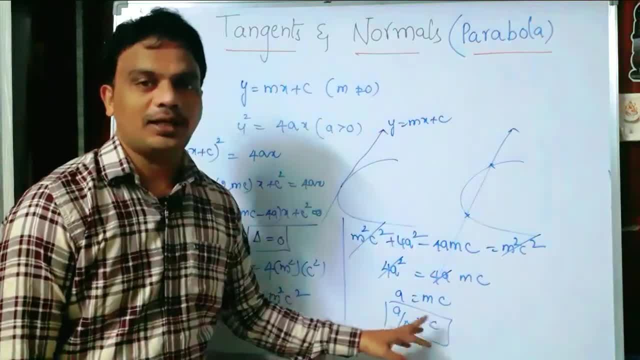 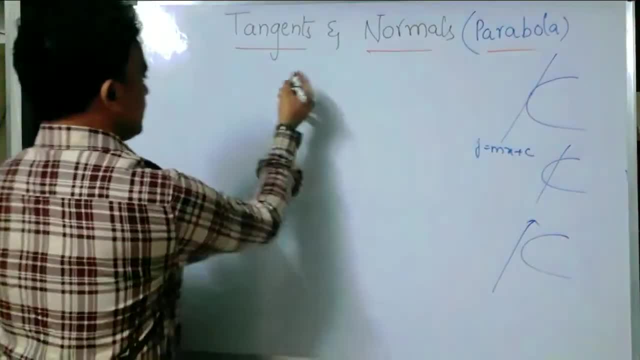 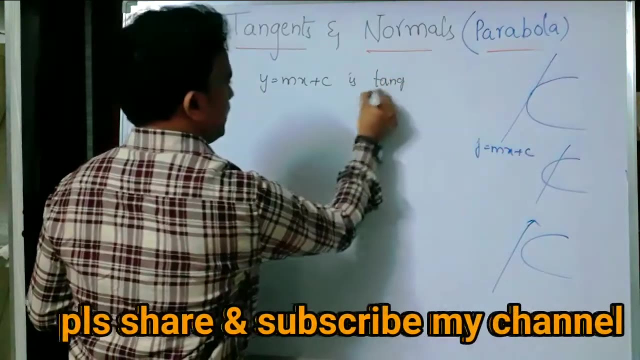 then what is your condition? C equals to a by m. Okay, so that will be the condition. So come on, students make a note. Okay, yes, So we got the condition. So y equals to mx plus c is a tangent, Okay. 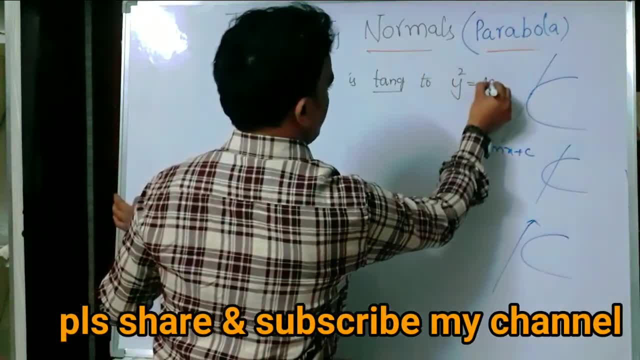 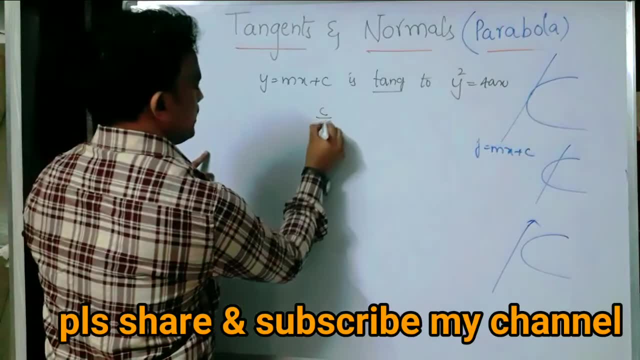 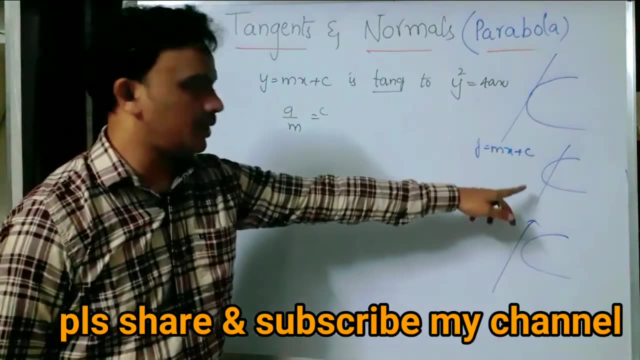 is a tangent to the parabola, y square is equals to 4ax. Okay, if it is a tangent, that means which touches the parabola. in that first case I got the condition. c equals to a by m. Okay, that is So if it intersect the parabola, if it intersect the parabola, we can get the. 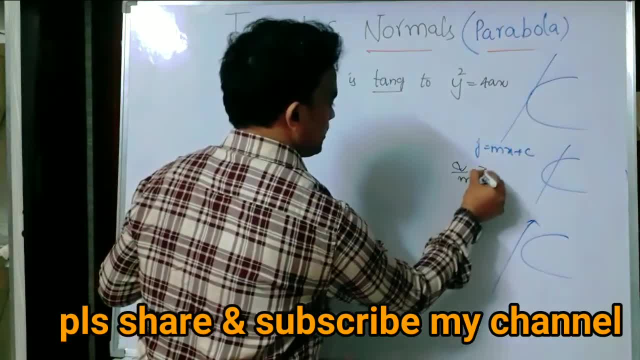 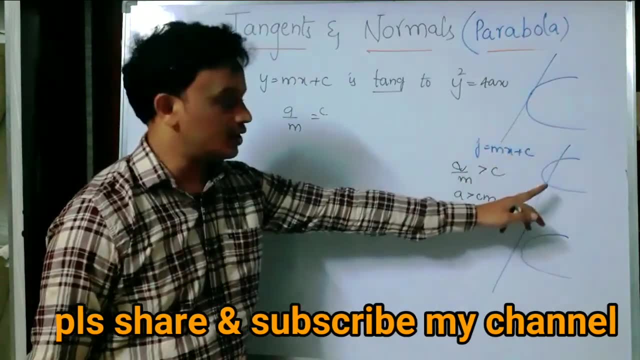 condition is so it is a by m is greater than c, that means a greater than c by m, In that case delta. just I have explained that. So delta should be greater than 0. So a by m greater. 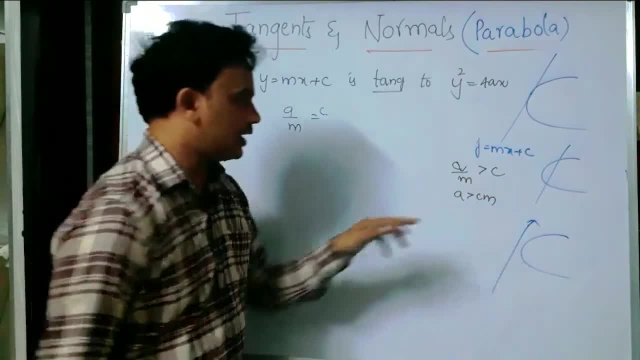 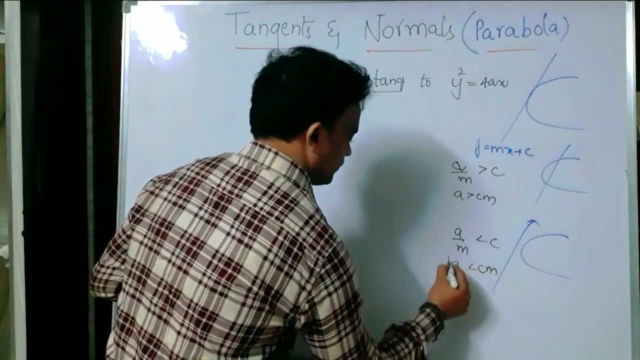 than 0. So a greater than c into m In that case. so a by m is less than c. that means a less than c into m. Okay, Okay, these are all the three conditions. So when the given line y equals to mx plus c, 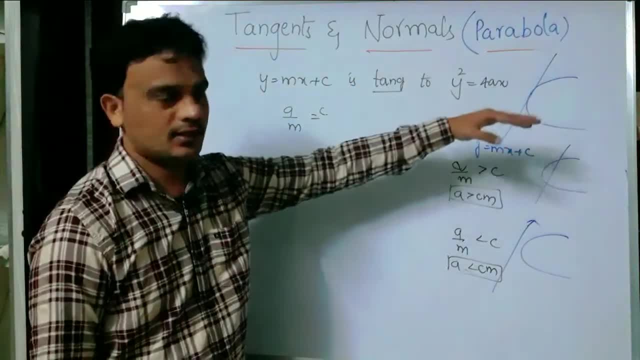 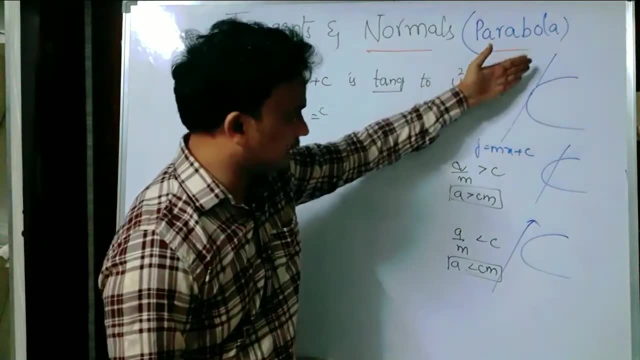 and to the parabola, y square is equals to 4ax, And so we are focusing on that. what is the condition for a tangent? when it becomes a tangent? Okay, that means so their point of intersection, this is not point of which it touches. So in that case, the second degree. 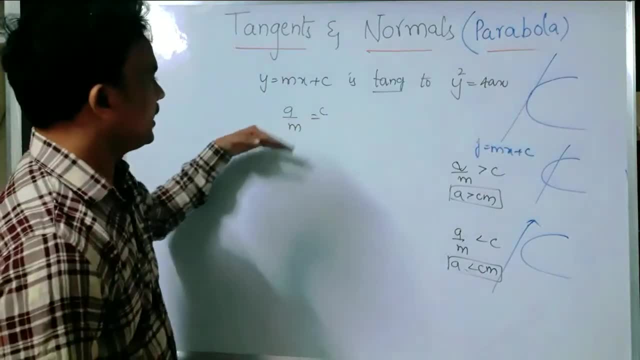 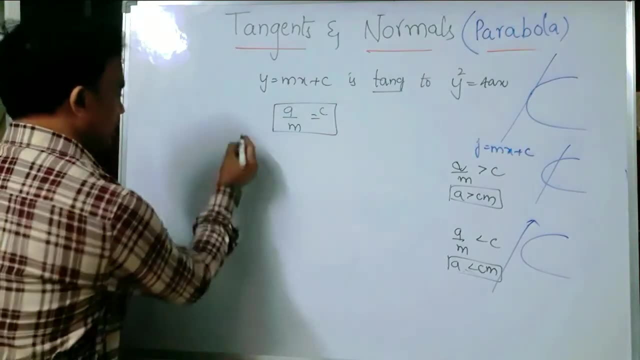 equation whose roots are equal. So I can get: the delta is equals to 0, then a by m equals to c is equals to a by m. So this is one of the important condition. Okay, Then in that case the tangent becomes. can I write the tangent: is y equals to mx plus what is? 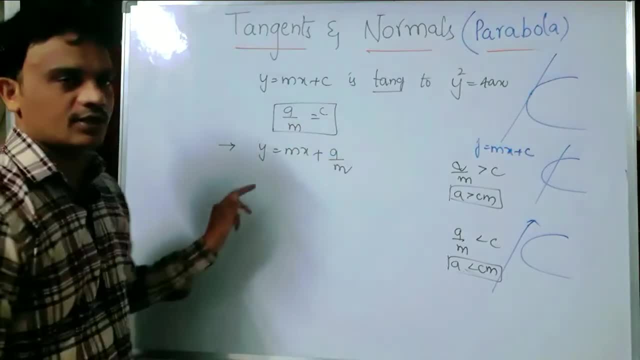 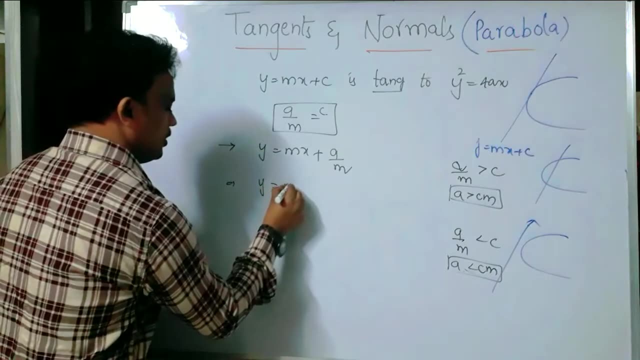 the c value a by m. Okay, So this is the equation of the tangent: y equals to mx plus a by m. Okay, Yes, by simplifying this one y equals to: it is m square x plus a by m, So that will be. 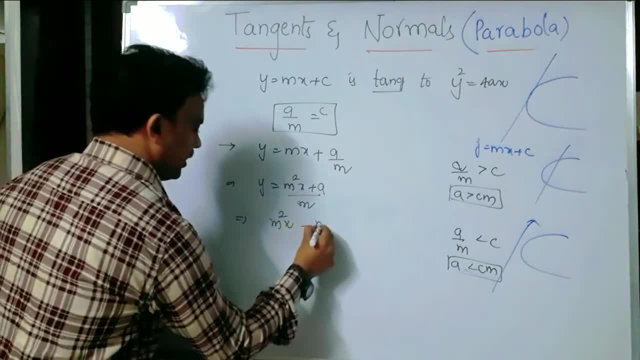 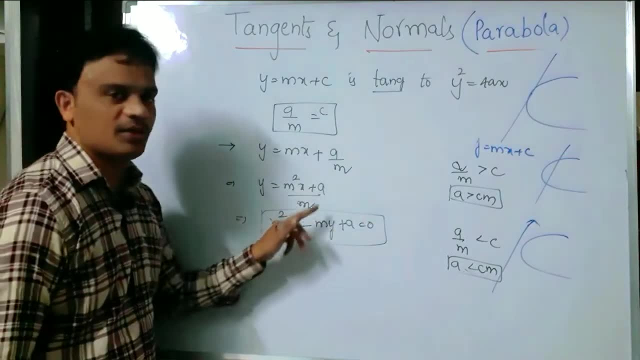 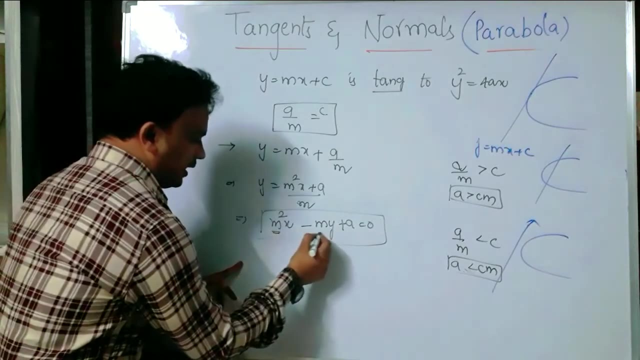 written as: m square x, okay, minus m into y plus a equals to 0.. Yes, please observe this condition: m square x minus my plus a equals to 0.. Here it is a second degree equation in terms of m's. please observe this one: m square and m and. 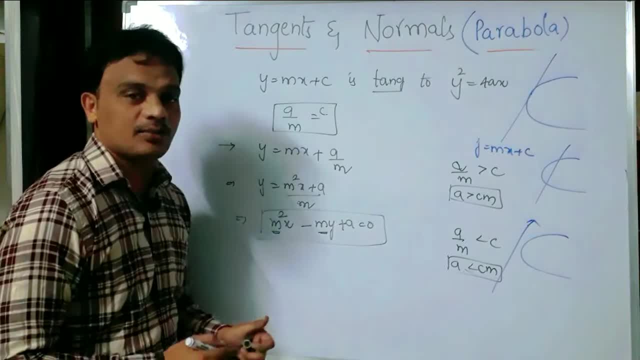 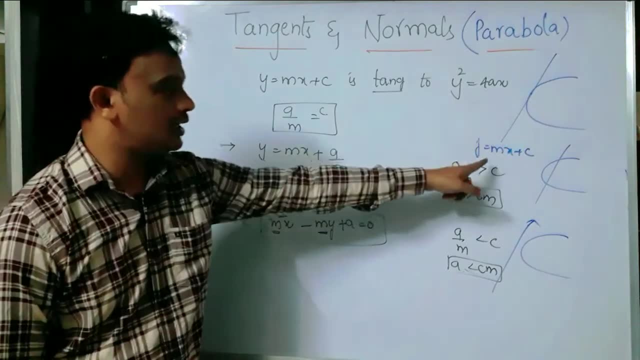 constant. Okay, it is a second degree equation in terms of m's. Okay, that means if y is equals to mx plus c is a tangent where m is the slope of the tangent. am I right or not? m is the slope. 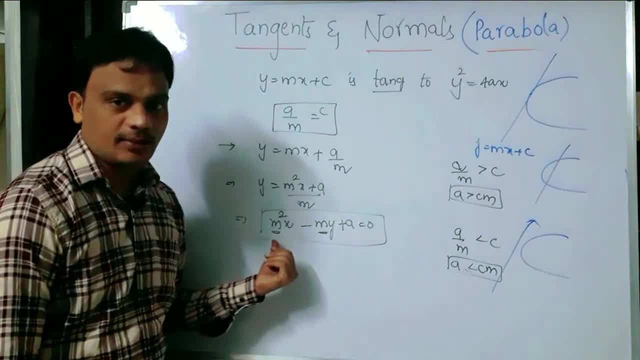 of the tangent. That means here you got that. two values for m, So two values for m. m has two values. So here m is the slope of the tangent, So here m is the slope of the tangent. So here. 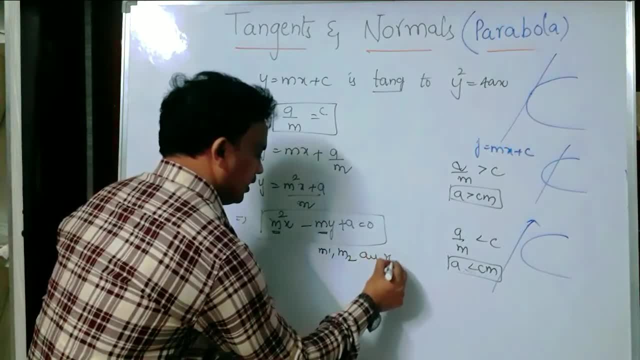 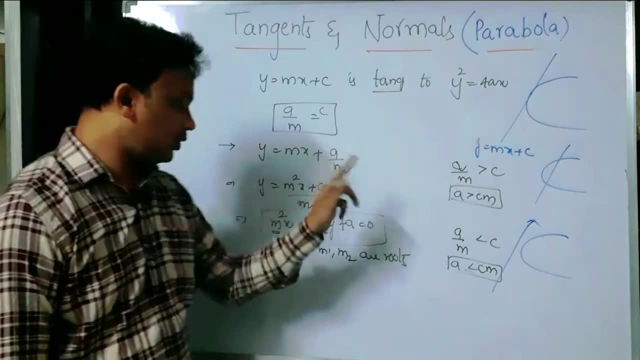 m1, m2 are the roots. m1, m2 are the roots of this equation. At the same time, what are m's are actually Slope of the tangents. Then you can decide this one. You can decide what you can. 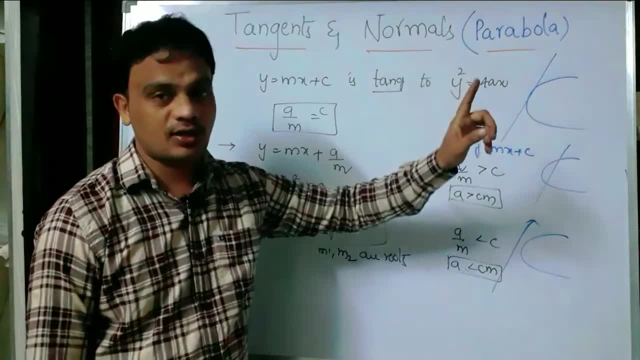 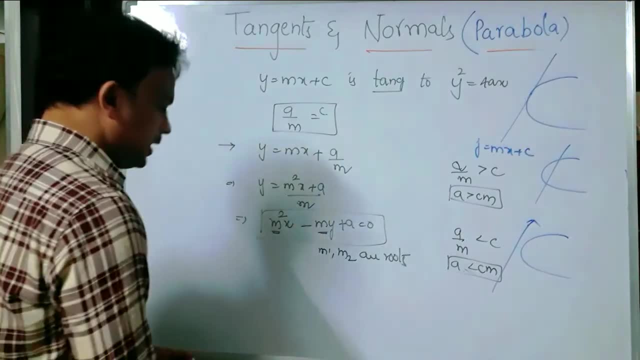 decide. So for the given parabola, you are going to draw the two tangents Here. you got the two values for slope, right or not? That means you can say: one more thing is the, you can get the. 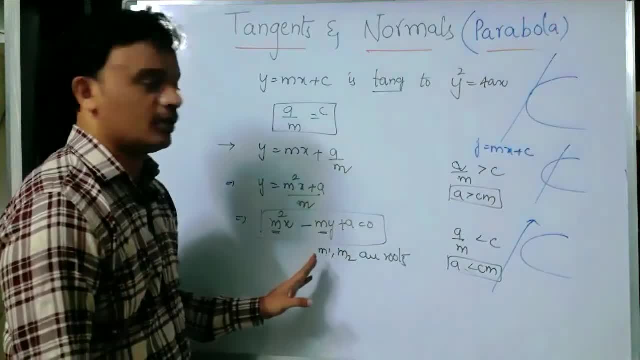 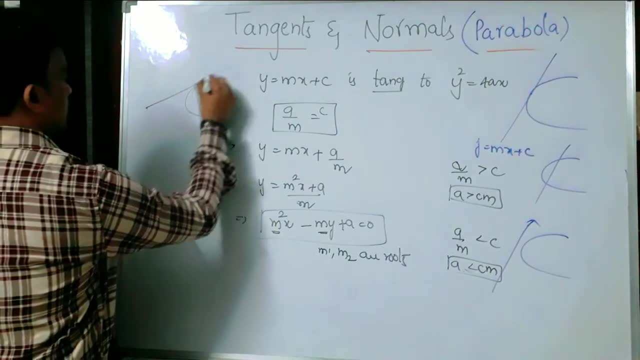 two tangents, two tangents whose slopes are m1 and m2 for the given parabola. So you can decide parabola. yes, like this. I can say So from an exterior point. we are going to get the two. 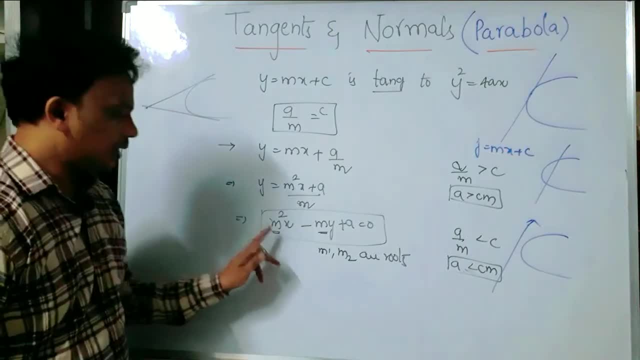 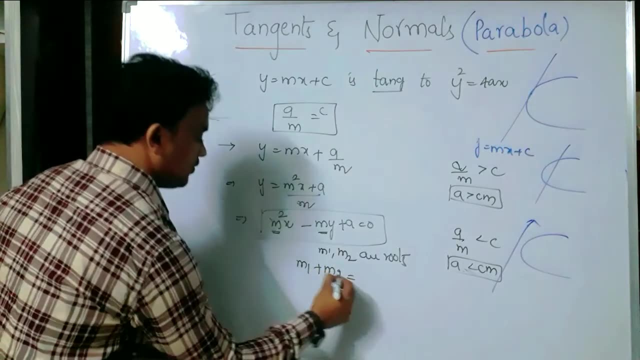 tangents. okay, whose slopes are m1 and m2, okay, Yes, from this one we can say one more thing: okay, Some of the roots, some of the slopes, I mean some of the slopes is so it is minus b. 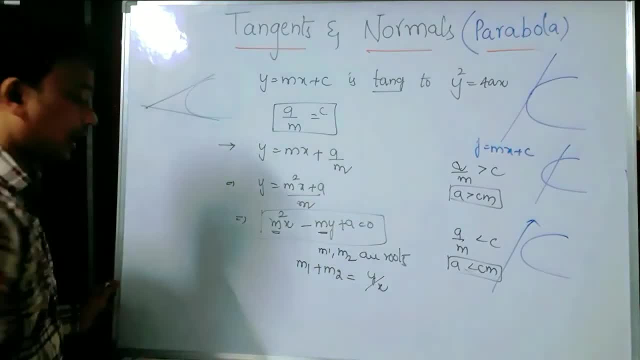 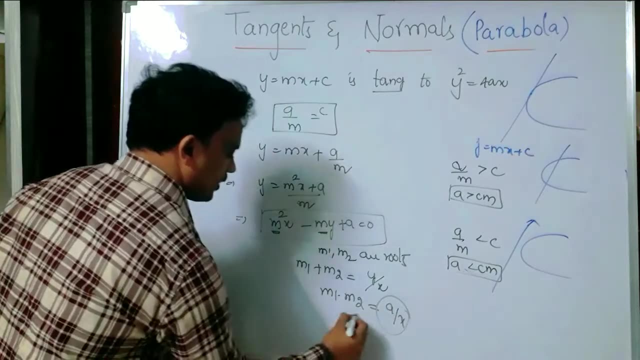 by a, which is y by x, And product of the slopes: m1 into m2,. m1 into m2 is a by x, m2 is a by x. okay, Yes, let us see. From this one I am going to get one more concept. 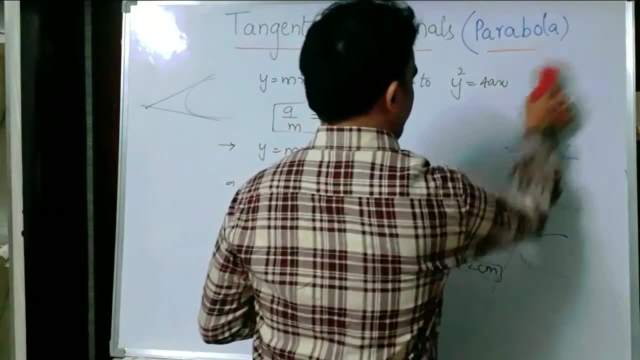 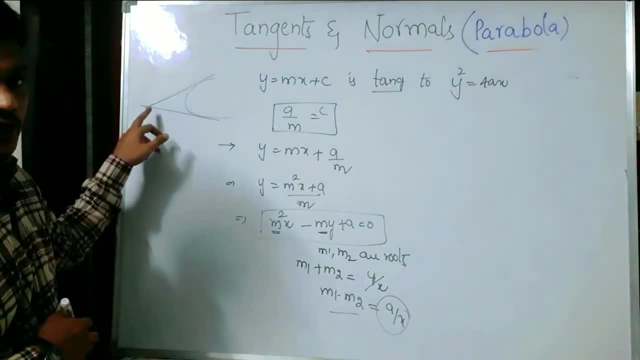 So what is the one more concept? Let us see What the thing is So actually. so I have drawn that two tangents. I can draw the two tangents from an exterior point to the parabola. So whose slopes? 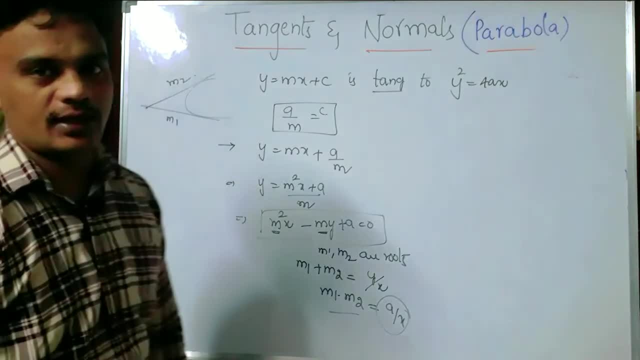 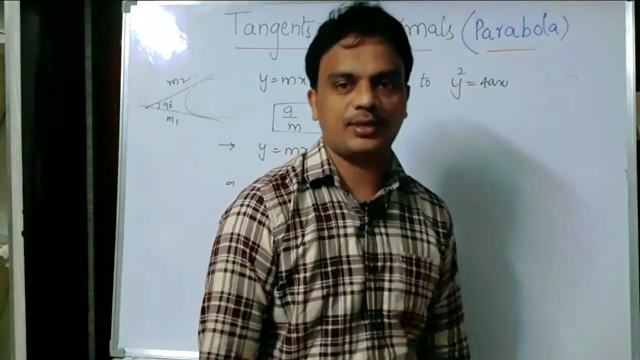 are m1 and m2, m1 and m2, okay, right, Okay, Now suppose if the angle between them is 90 degrees? between them is 90 degrees. So what is this location? What is the locus of point of intersection? 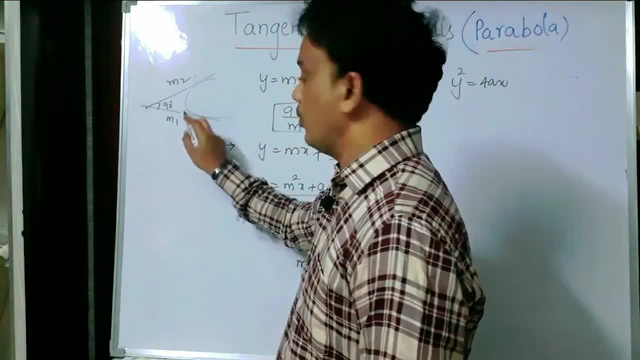 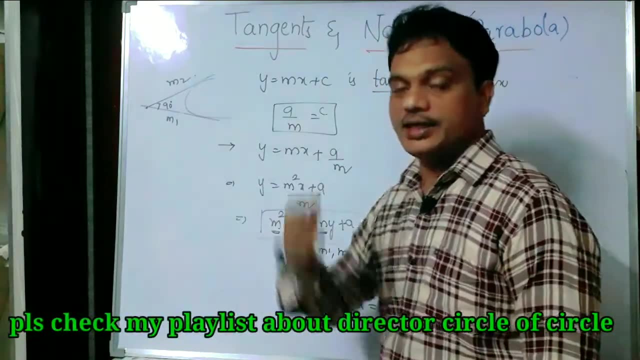 of the tangents which are drawn from an exterior point. Which are? which type of tangents? Perpendicular tangents, perpendicular tangents. So what is the location? Okay, In case of circle, in case of circle, we can get a direct circle. Please remind this one In case of a circle. 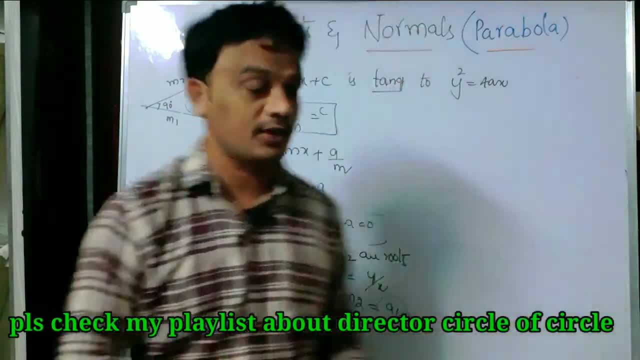 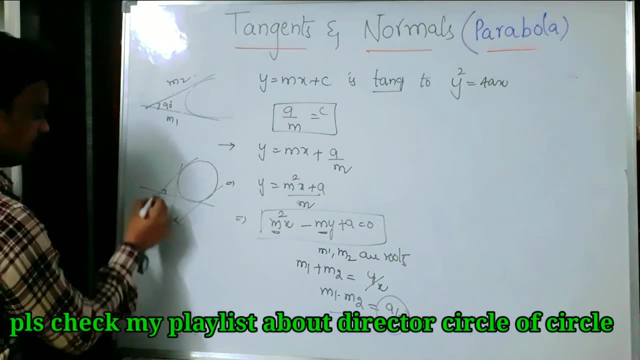 the locus of point of intersection of perpendicular tangents to the circle, right? Do you remember that one? Okay, So here, that 90 degrees angle between them is 90 degrees. we can get a circle. In case of a circle, that is called a. 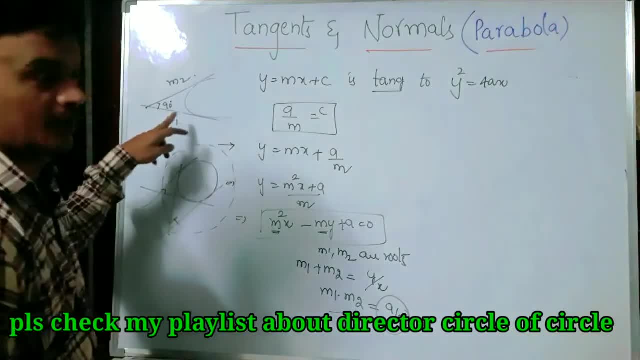 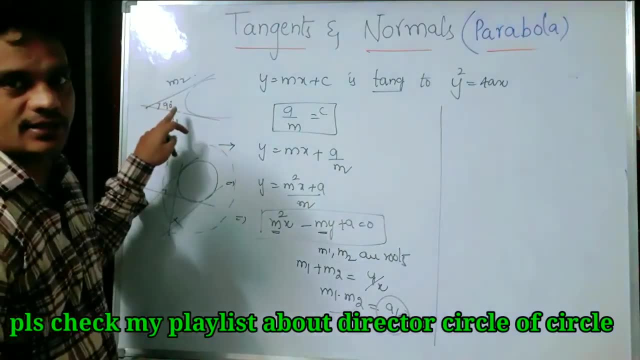 director cycle. But what will happen In case of parabola? let us see: Okay, Yeah, So if they are 90, angle between them is 90 degrees, okay, then product of the slopes is equals to minus 1,. 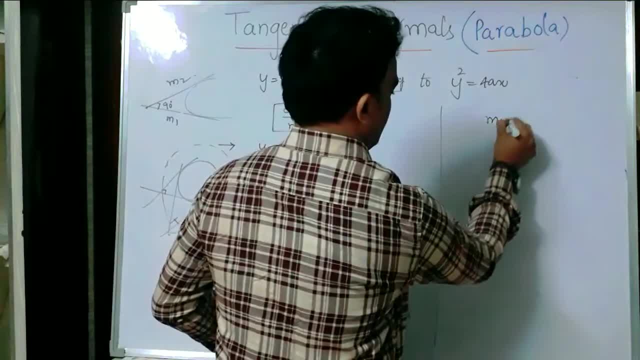 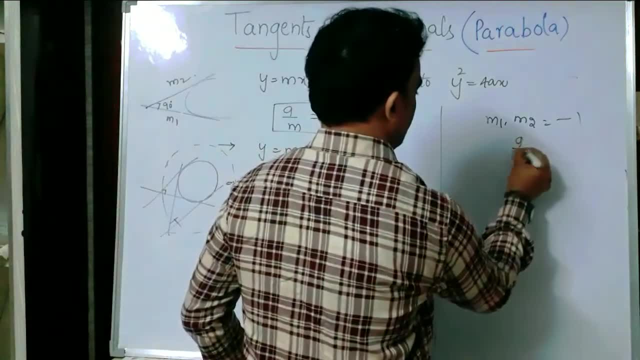 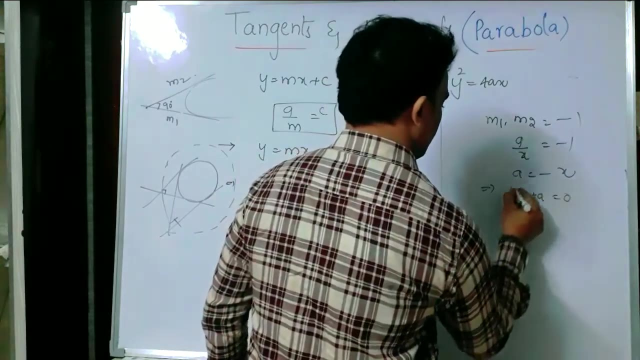 am I right or not? Product of the slopes is minus 1.. Then I can say: m1 into m2 equals to minus 1.. So actually, what is m1 into m2? a by x? a by x is equals to minus 1.. a equals to minus x. I can write: x plus a equals to 0. 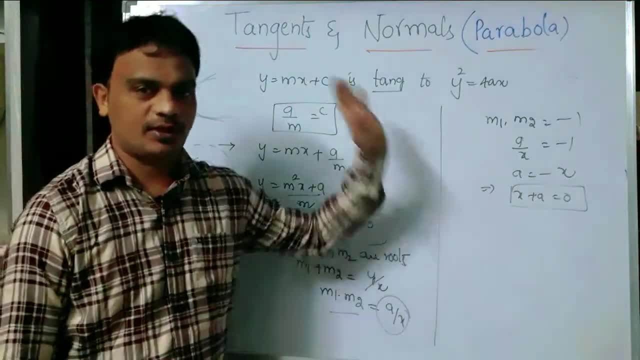 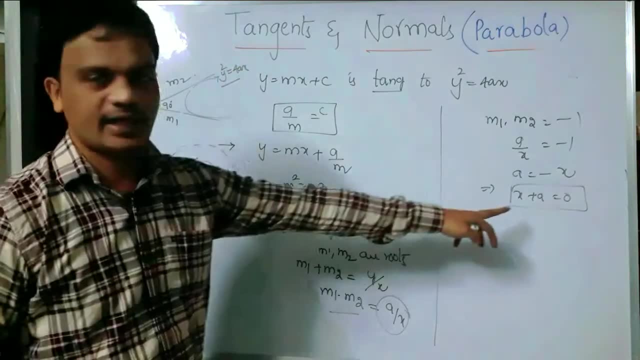 x plus a equals 0.. What is x plus a? actually, From the standard form of the parabola? for y square is equals to 4ax. For y square is equals to 4ax. what is x plus a? So? 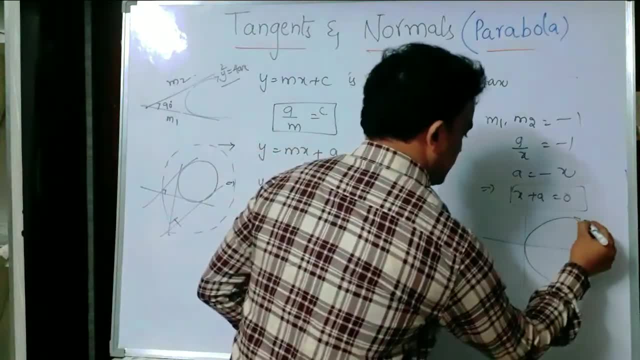 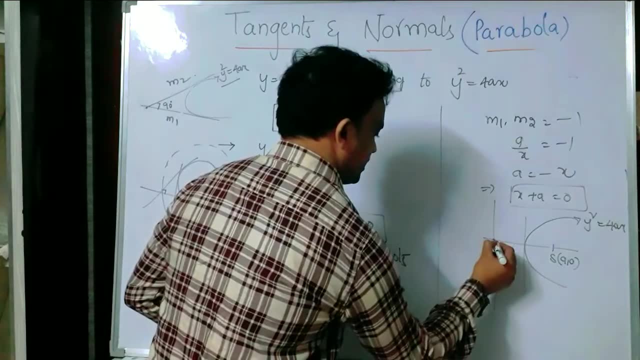 can I remind you for this one? So y square is equals to 4ax. So s is the focus, a comma 0.. This will be the directrix. This point is z minus a comma 0.. And what is the equation of the? 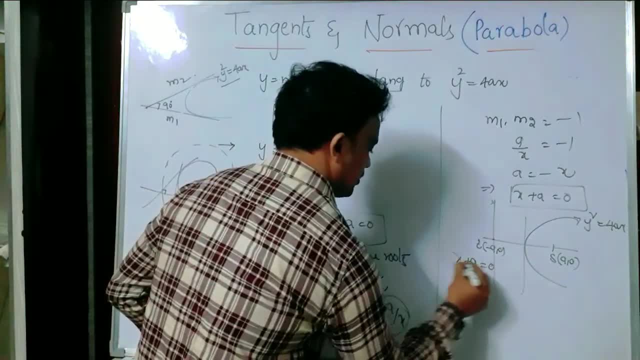 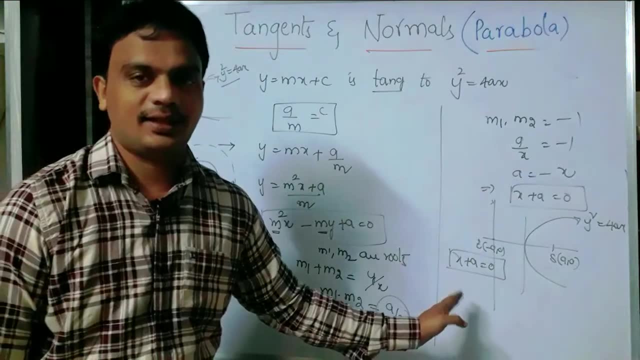 directrix is: x plus a is equals to 0.. x plus a is equals to 0. Then what is that location Will be the directrix. That means what is the final conclusion? is the so from the directrix. 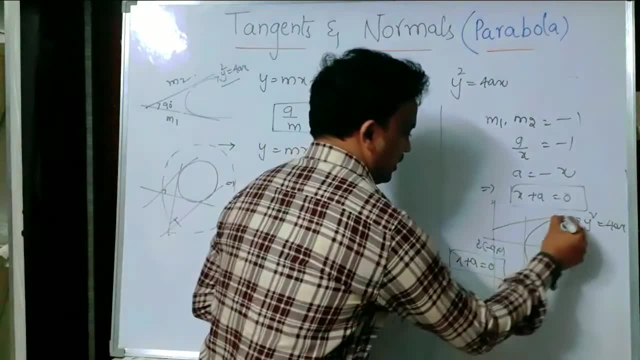 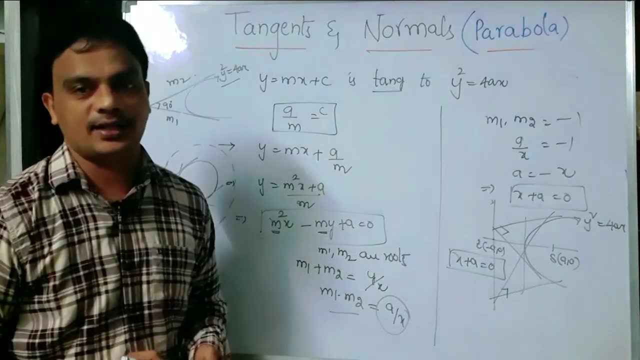 from the directrix if you are going to take any point. so you are going to draw the tangents. you are going to draw the tangents. What is the angle between is 90 degrees. okay, so conclusion which is so parabola, key tangents, exterior points to draw. 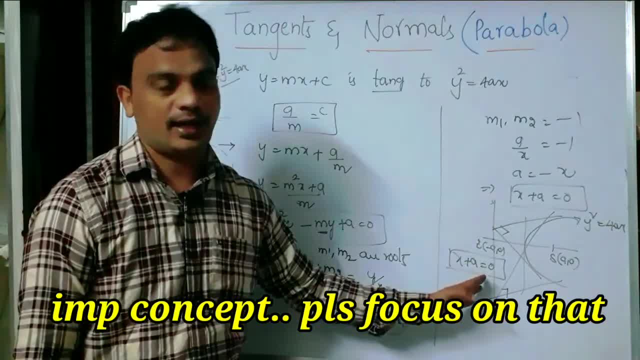 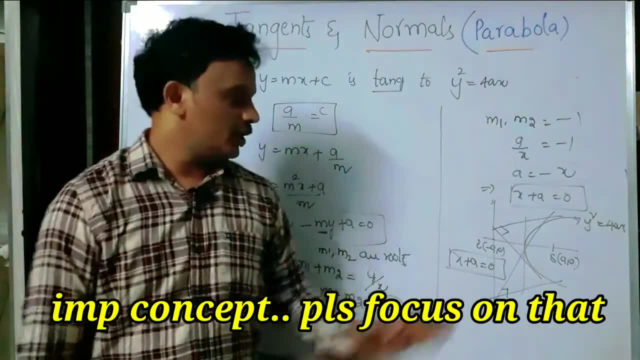 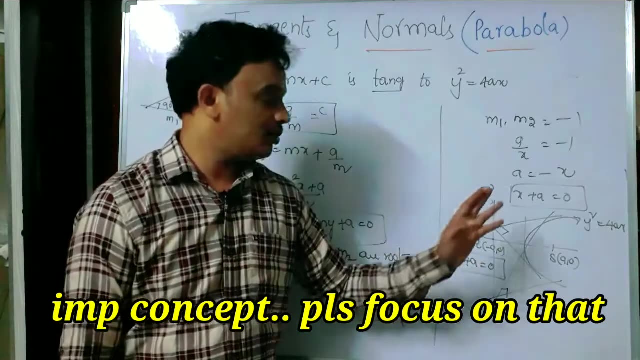 what much? angle? 90 degrees from the end day. angle 90 degrees from the end day compulsory. that point lies on direct rigs, right? or else you can say: conversely, if you are going to take any point on the direct rigs and drawn to the two tangents to the parabola, the angle between them must be: 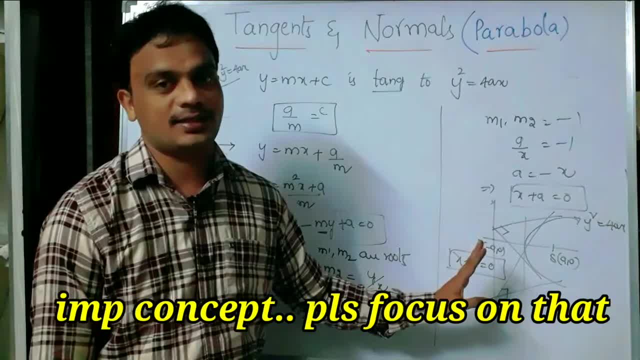 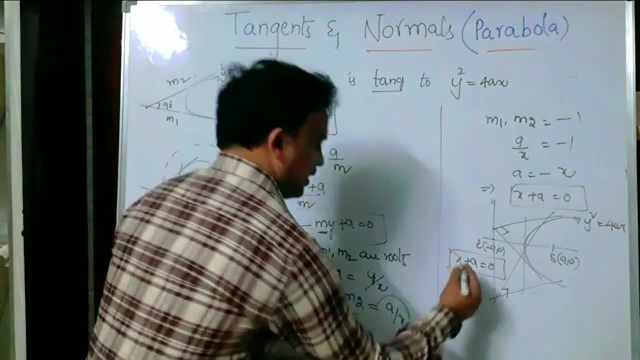 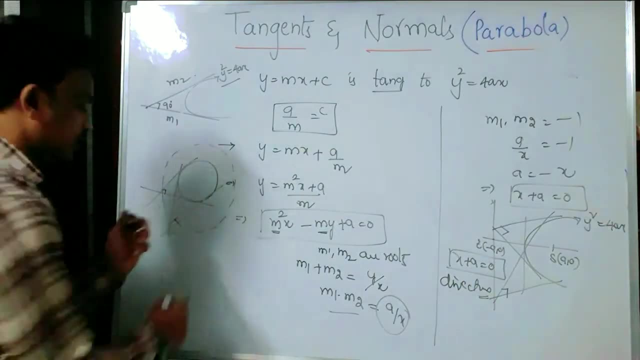 90 degrees. so that will be the very important case. okay, so what is the locus of point of intersection of perpendicular tangents to the parabola means what you can say, which is the direct rigs, okay, but in case of circle, in case of circle, you can get that circle. so which is? 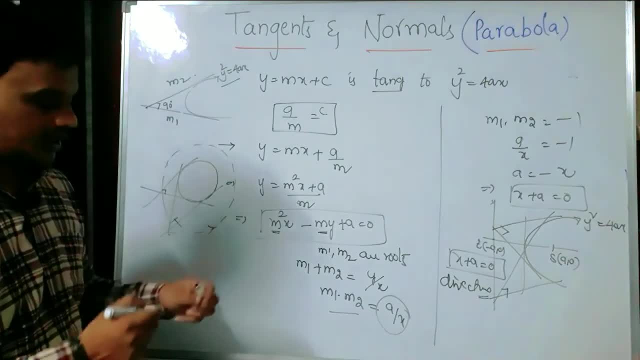 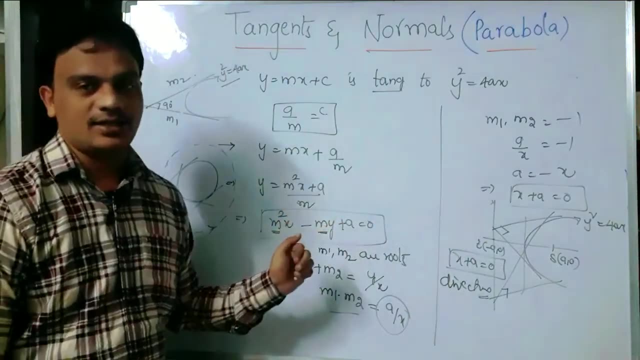 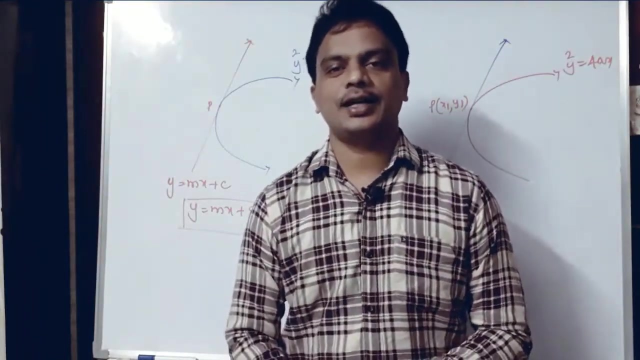 called here in this case, which is called a director circle. okay, in that case, suggest we got a line. what is the line? is the direct rigs. so so, in the objective point of view, very important condition. okay, next, yes, come on, students, make a note. okay, students, so that is about the condition for that. a line y is equals. 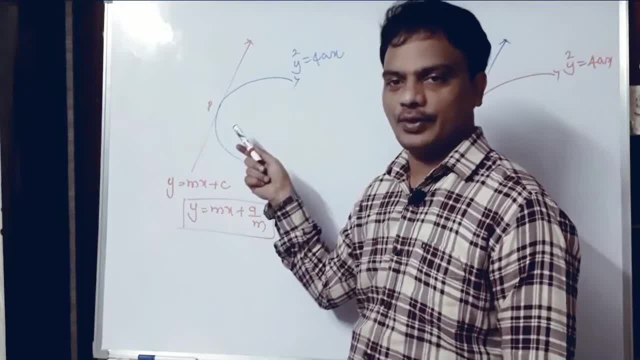 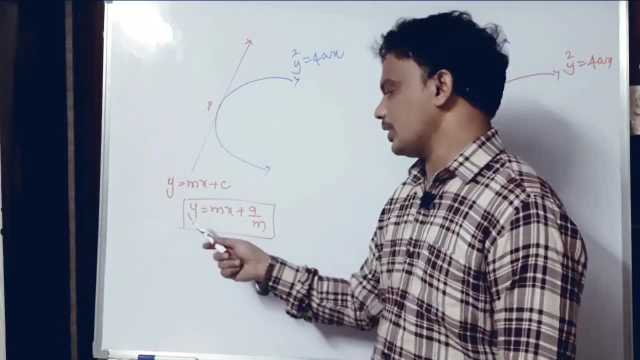 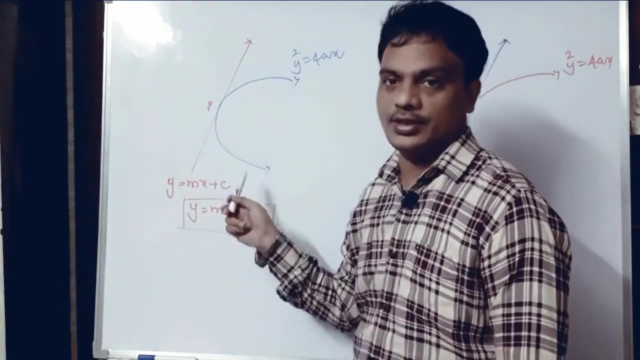 to mx plus c is given when it becomes a tangent. okay, so y equals to mx plus c is a tangent. what is the condition? so c is equals to a by m. then we can get that. what is the equation of a tangent? so y is equals to mx plus a by m. so when one line is given, so this condition is a. when one line y.